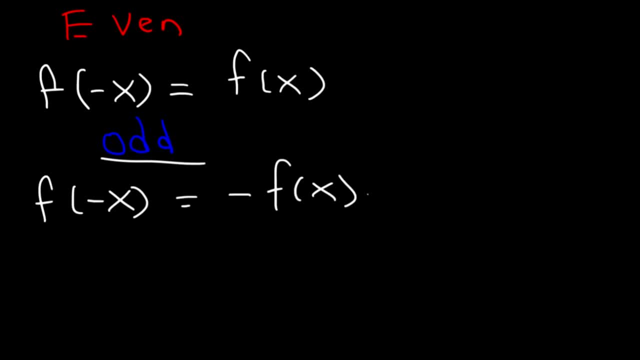 Everything in the function has to change sign. If one term changes sign and the rest do not, it's not going to be odd. Now what about the last category? When is a function? neither even nor odd. It's going to be neither if you plug in negative x and if you do not get negative f of x. 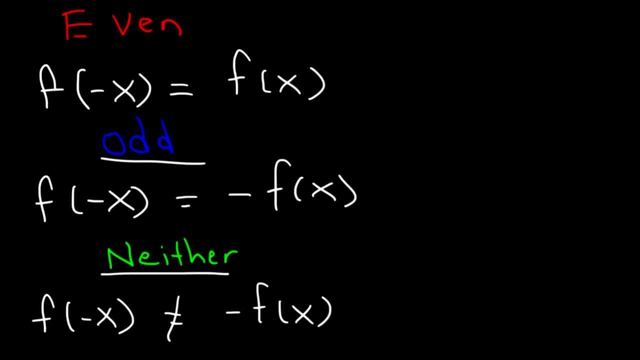 So what does that mean? Well, let's say, if you replace x with negative x and some signs change while others don't, then it's going to be neither. Also, if it doesn't equal f of x, too, it's also neither. 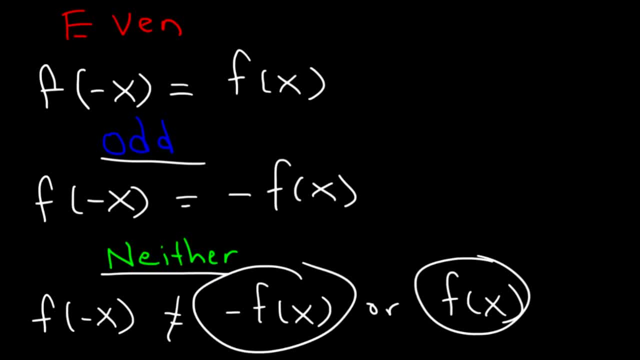 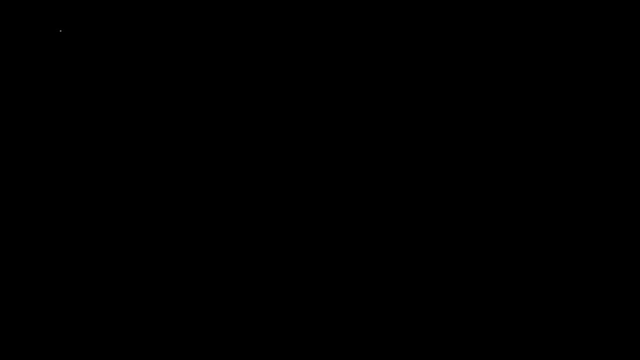 So it can't equal negative f of x or f of x. So, basically, as long as it's not even or odd, it's neither. So let's start with. Let's start with our first example. Let's say that f of x is equal to x, to the fourth plus 3x squared. 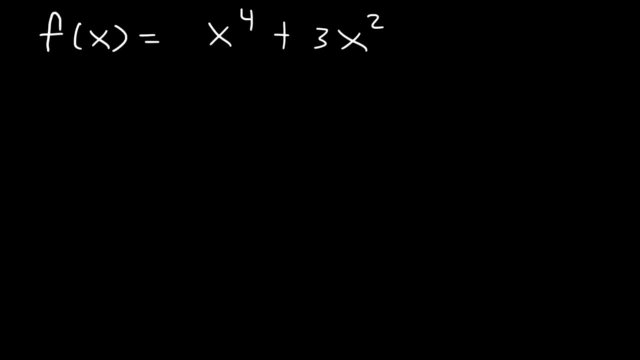 So is the function even, odd, or is it neither? Well, here's how you do it, the easy way: Look at the exponents. Is 4 even or odd? 4 is an even number. Now what about 2?? Is it even or odd? 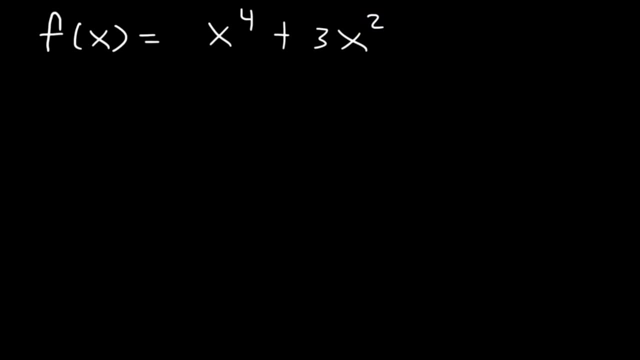 2 is even. So if all the exponents are even, then the function is going to. It's going to be even. But now let's prove it. Let's show our work. Let's replace x with negative x. So this is going to be negative x raised to the fourth power plus 3 times negative x squared. 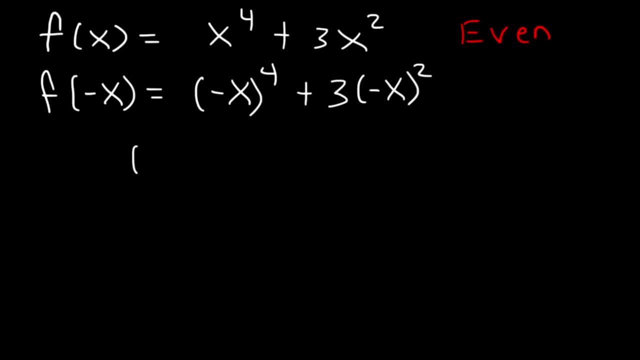 Now what is negative? x raised to the fourth power, That's basically negative. x times itself four times Negative. x squared is negative. x times itself two times. Two negatives is a positive. Three negatives will give you a negative result, but four negatives will give you a positive result. 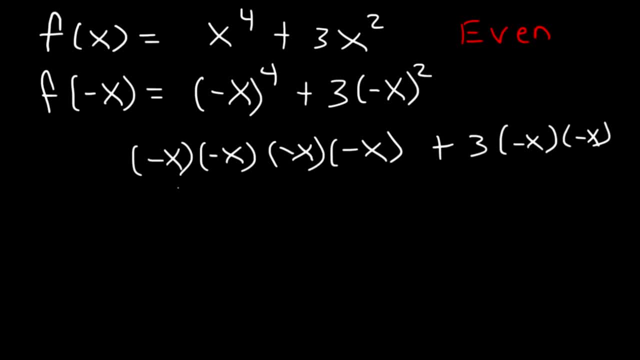 Anytime you have an even number of negative signs, it's going to produce a positive sign. So this is going to be positive. x to the fourth plus 3x squared, Two negative signs will produce a positive result. Now notice that the function that we have is the same as the original. 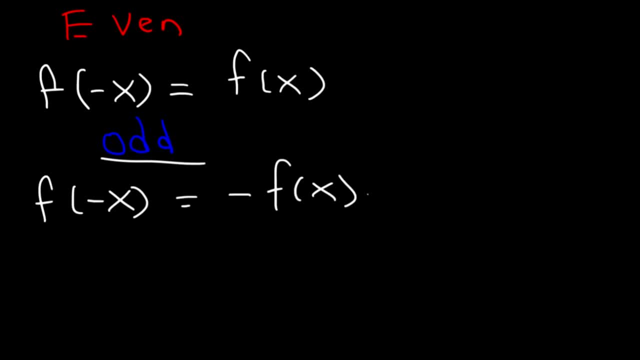 Everything in the function has to change sign. If one term changes sign and the rest do not, it's not going to be odd. Now what about the last category? When is a function? neither even nor odd. It's going to be neither if you plug in negative x and if you do not get negative f of x. 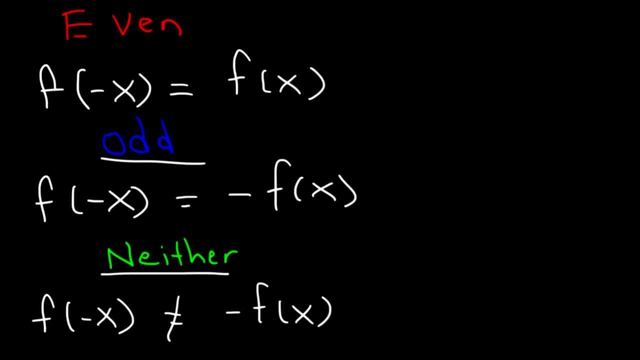 So what does that mean? Well, let's say, if you replace x with negative x and some signs change while others don't, then it's going to be neither. Also, if it doesn't equal f of x, too, it's also neither. 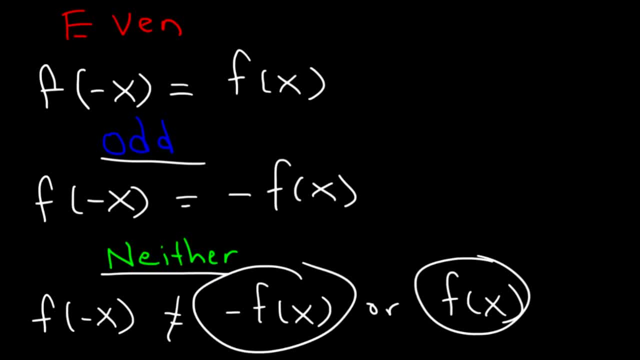 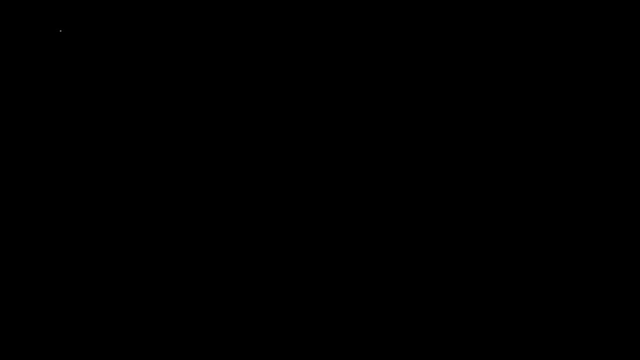 So it can't equal negative f of x or f of x. So, basically, as long as it's not even or odd, it's neither. So let's start with. Let's start with our first example. Let's say that f of x is equal to x, to the fourth plus 3x squared. 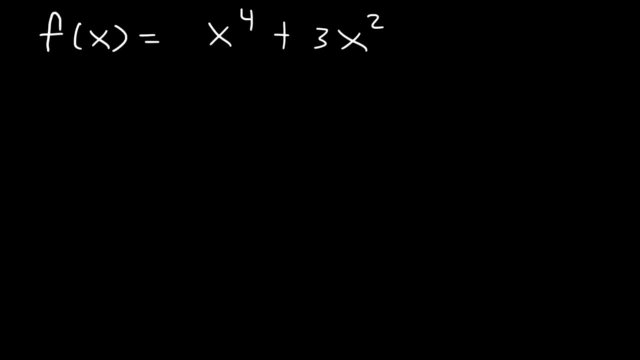 So is the function even, odd, or is it neither? Well, here's how you do it, the easy way: Look at the exponents. Is 4 even or odd? 4 is an even number. Now what about 2?? Is it even or odd? 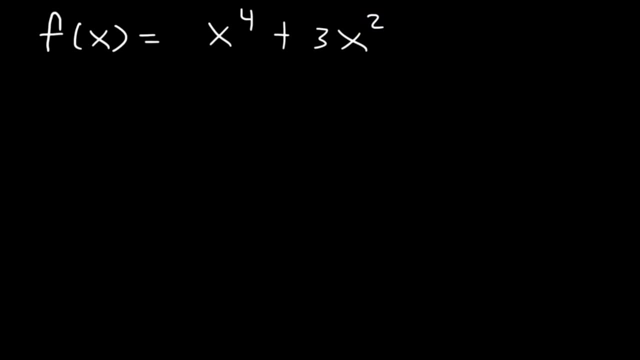 2 is even. So if all the exponents are even, then the function is going to. It's going to be even. But now let's prove it. Let's show our work. Let's replace x with negative x. So this is going to be negative x raised to the fourth power plus 3 times negative x squared. 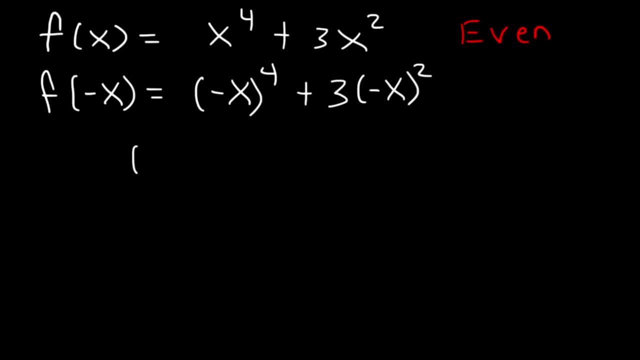 Now what is negative? x raised to the fourth power, That's basically negative. x times itself four times Negative. x squared is negative. x times itself two times. Two negatives is a positive. Three negatives will give you a negative result, but four negatives will give you a positive result. 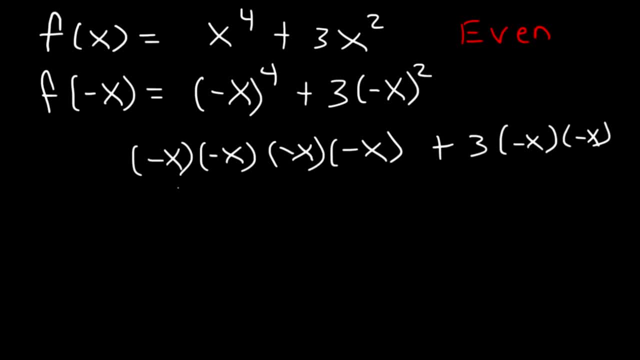 Anytime you have an even number of negative signs, it's going to produce a positive sign. So this is going to be positive. x to the fourth plus 3x squared, Two negative signs will produce a positive result. Now notice that the function that we have is the same as the original. 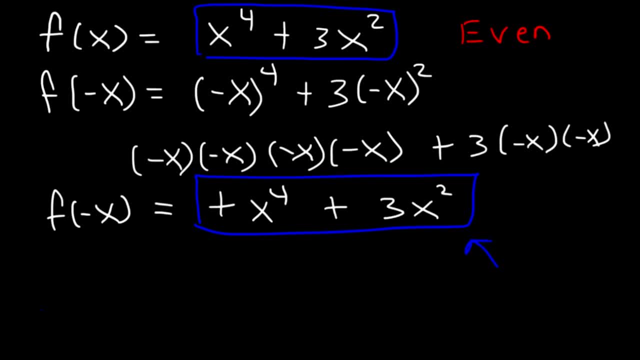 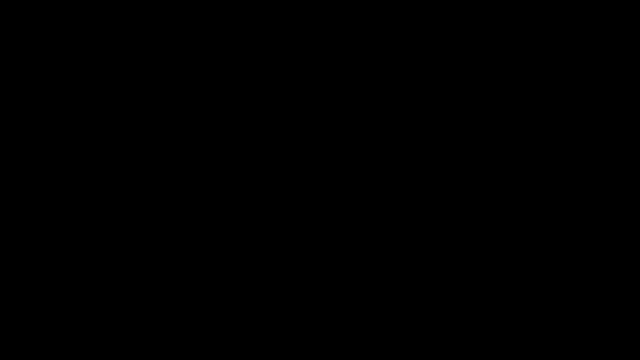 Therefore, this is equal to f of x. So we can make the statement that f of negative x is equal to f of x, which is the definition of an even function. Now let's try our next example. Let's say that f of x is equal to x to the fifth power, plus 2x to the third power. 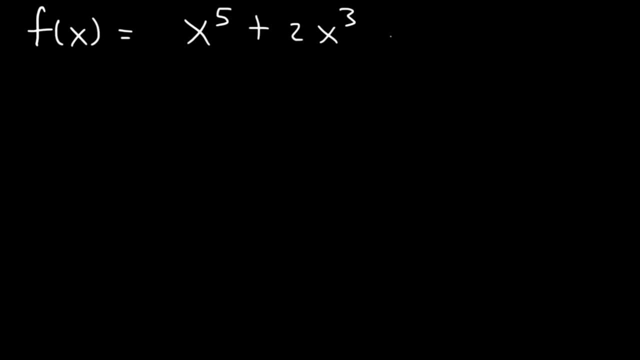 Is it even Odd Or neither? Now, don't worry about the coefficient, This is unimportant. Even though 2 is an even number, that's not going to help us determine if it's even or odd. Look at the exponent. 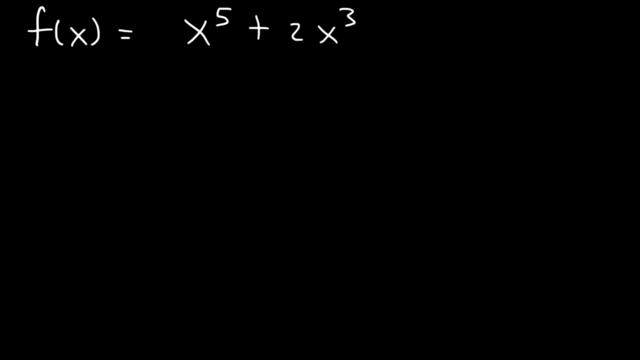 Five. is it even or odd? Five is an odd number And three is also an odd number. Since all of the exponents are odd, the function is going to be an odd function. And now let's prove it. Let's replace x with negative x. 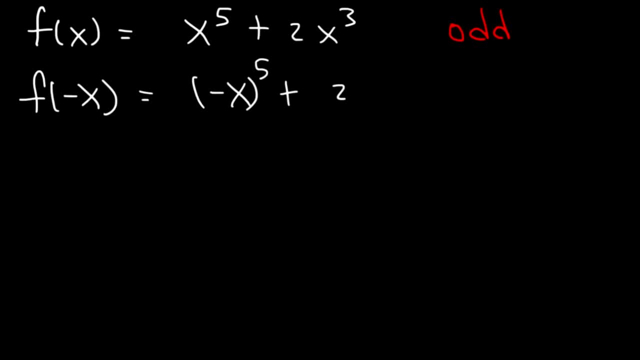 Now, whenever you have an odd number of negative signs, the result will be negative. For example, negative x to the third power. Negative x times negative. x is positive x squared times another negative x, That's negative x cubed. So this is going to be negative x to the fifth power minus 2x cubed. 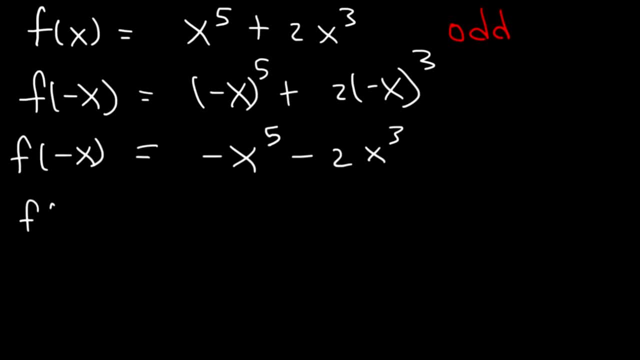 And all of that is equal to f of negative x. Now, what should we do in our next step In order to prove that this function is an odd function? What you want to do is you want to factor out a negative one. If you take out negative one, negative x to the fifth, divided by negative one, is positive. 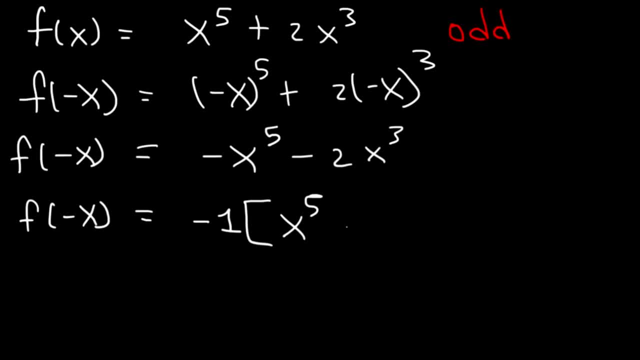 x to the fifth, All the signs will change. Negative 2x cubed will become positive: 2x cubed. Now notice that this portion inside the brackets, x to the fifth plus 2x cubed, is equal to the original function. 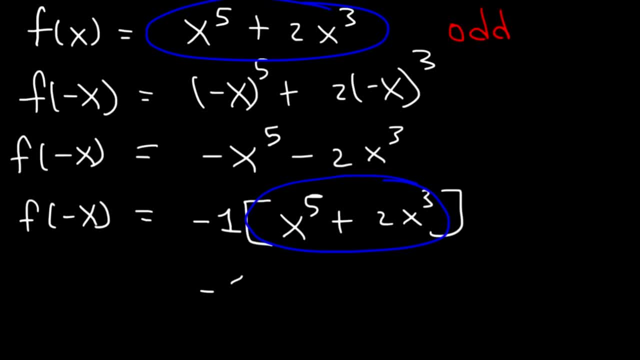 So at that point, what you want to do is replace it. So what you want to do is replace it With the original function, f of x. So therefore, we can say that f of negative x is equal to negative f of x, which is the. 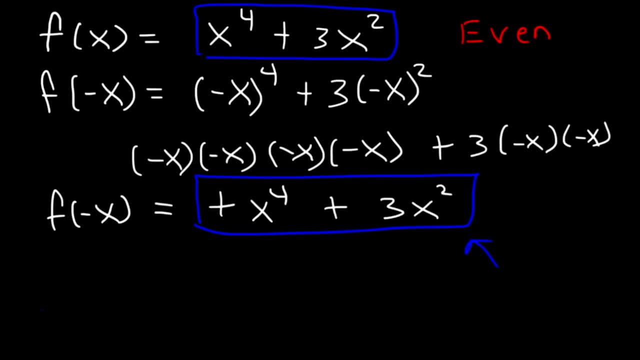 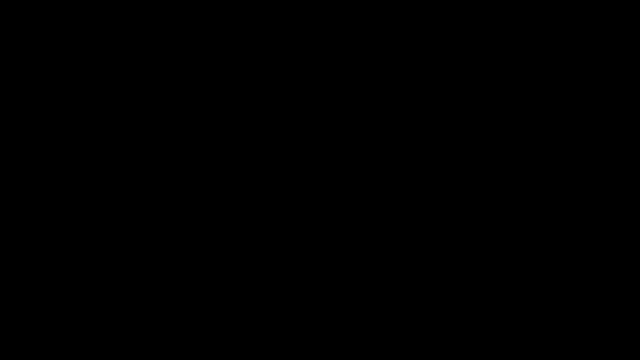 Therefore, this is equal to f of x. So we can make the statement that f of negative x is equal to f of x, which is the definition of an even function. Now let's try our next example. Let's say that f of x is equal to x to the fifth power, plus 2x to the third power. 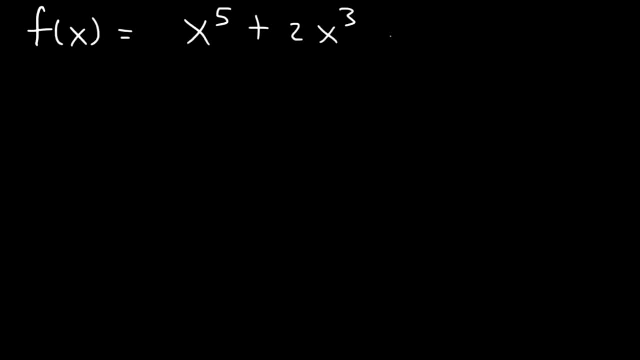 Is it even Odd Or neither? Now, don't worry about the coefficient, This is unimportant. Even though 2 is an even number, that's not going to help us determine if it's even or odd. Look at the exponent. 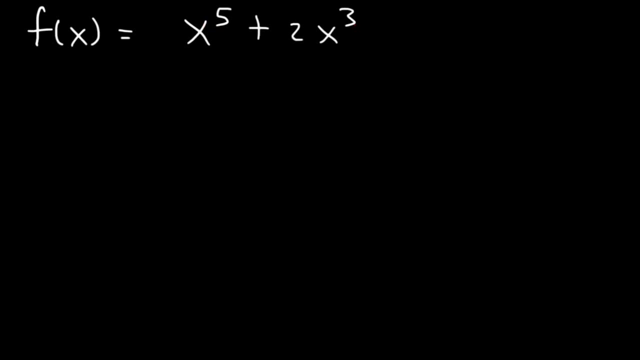 Five. is it even or odd? Five is an odd number And three is also an odd number. Since all of the exponents are odd, the function is going to be an odd function. And now let's prove it. Let's replace x with negative x. 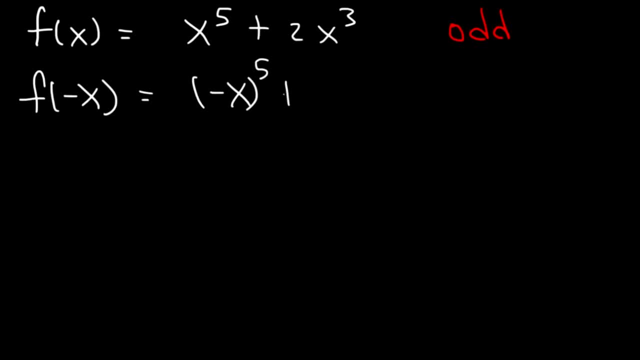 Let's replace x with negative x Now. whenever you have an odd number of negative signs, the result will be negative. For example, negative x to the third power. Negative x times negative x is positive x. squared times another negative x, That's negative x cubed. 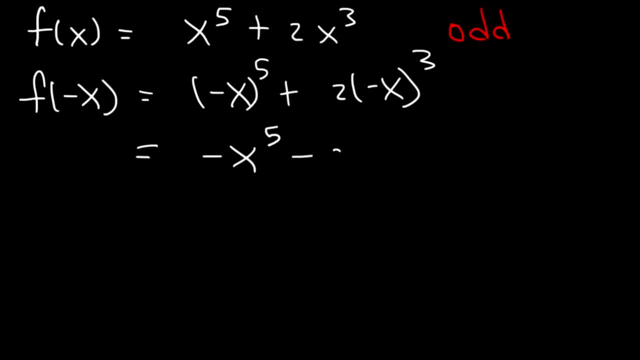 So this is going to be negative x to the fifth power minus 2x cubed, And all of that is equal to f of negative x. Now, what should we do in our next step? Well, first we'll take out the x to the third power, and all of it's always negative. 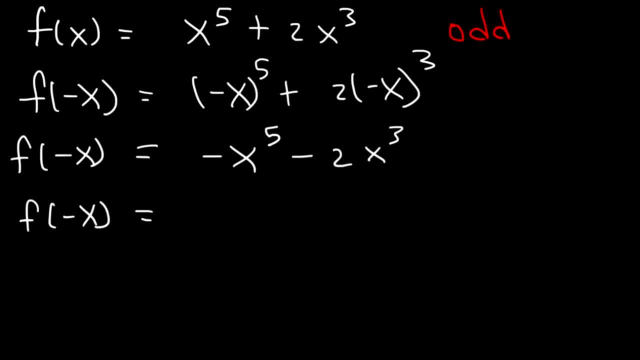 We're going to start by writing down the curve and the value of the curve in order to prove that this function is an odd function. What you want to do is you want to factor out negative 1.. If you take out negative 1, negative x to the fifth divided by negative 1 is positive. 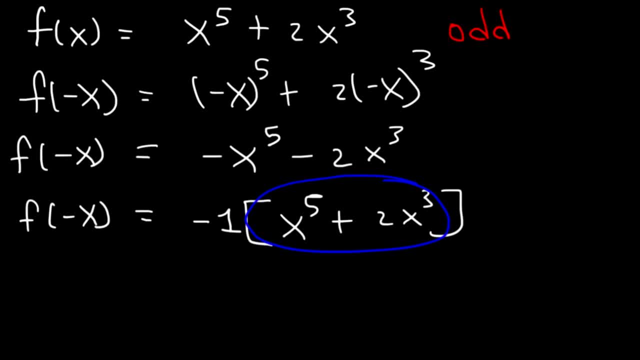 x to the fifth, All the signs will change. Negative 2x cubed will become positive 2x cubed. Now notice this portion Inside the brackets. X to the fifth plus 2x cubed is equal to the original function. 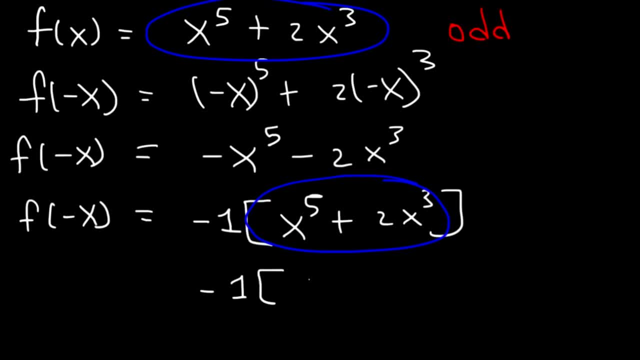 So at that point, what you want to do is replace it with the original function f of x. So therefore we can say that f of negative x is equal to negative f of x, which is the definition of an odd function. And that's how you can prove it. 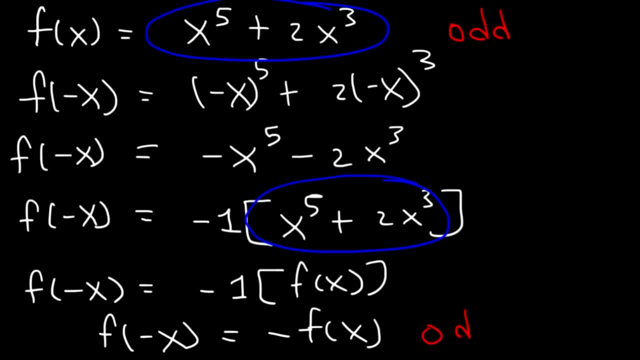 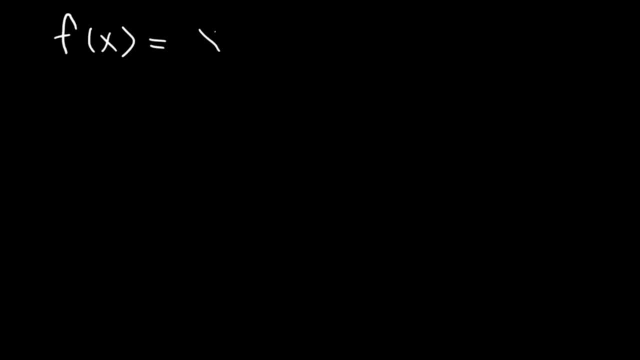 definition of an odd function, And that's how you can prove it. Now, what about this one? Let's say that f of x is equal to x squared plus 6. Is it even or odd? Well, you know, x squared is an even component. 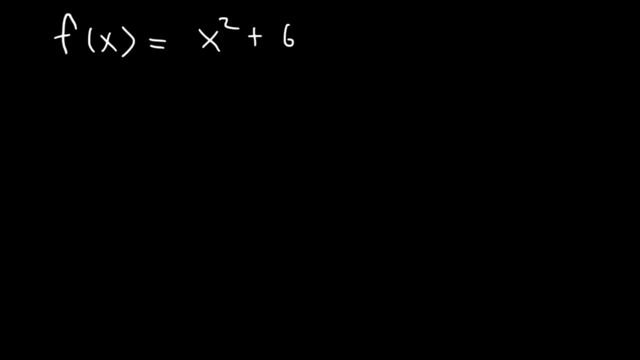 Because it has an even exponent. What about 6?? Well, 6 is the same as 6x to the 0.. Anything raised to the 0 power is 1.. So x to the 0 is 1.. Which 6 times x to the 0 is 6 times 1 at 6.. 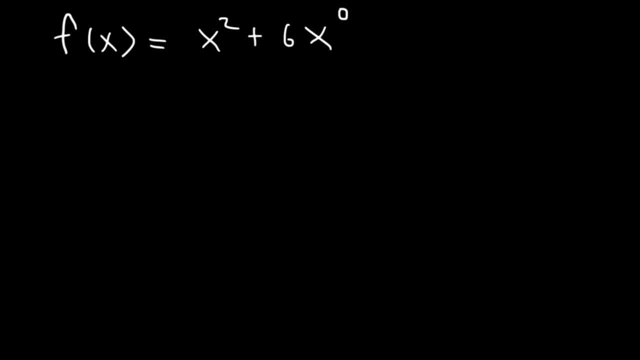 And 0 is an even exponent, So the whole thing is going to be even. So let's go ahead and prove it Now. let's replace x with negative x, So this is going to be negative x squared plus 6.. Negative x times negative x is positive x squared. 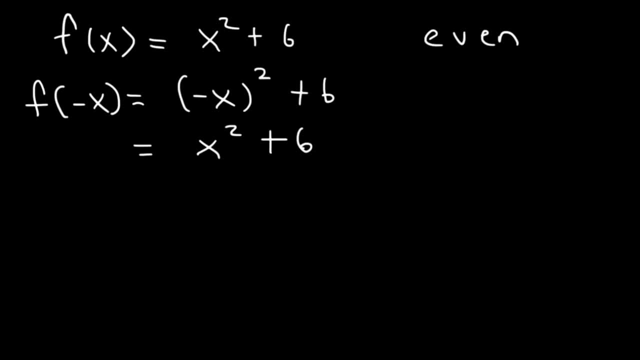 So we have x squared plus 6.. Notice that the function did not change. So on the right side we can replace x squared plus 6 with f of x. On the left side we still have f of negative x. So whenever f of negative x is equal to positive f of x, then it's an even function. 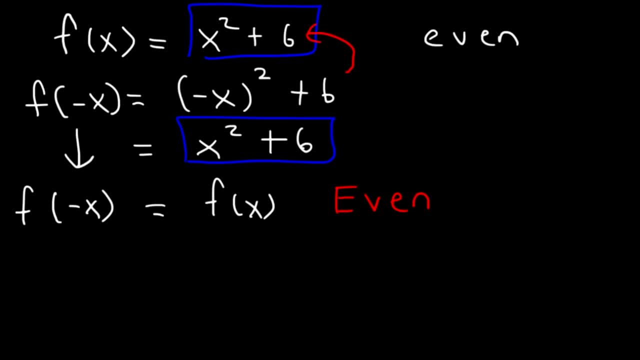 So if you see a number, it's even Think of that number as being multiplied times x to the 0.. And 0 is an even number, like 2, 4, 6.. What about x cubed minus 8x? 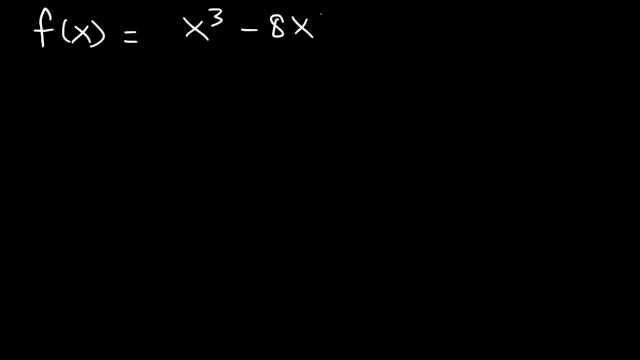 Is that even or is it odd? Well, whenever you see an x, it's basically x to the first power. Now, 1 and 3 are odd numbers. So therefore, this is an even function. This is going to be an odd function. 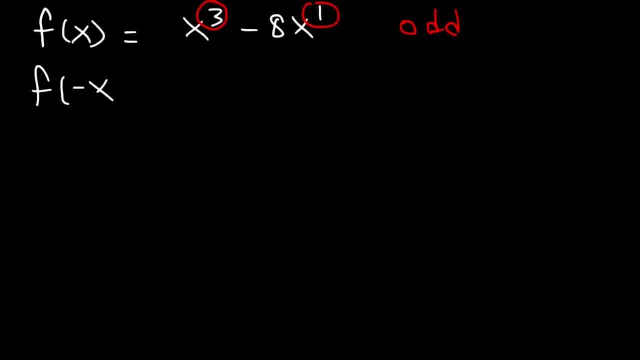 Now let's prove it. So let's find f of negative x. This is negative x to the third power minus 8 times negative x. Negative x to the third power is negative x. cubed Negative 8 times negative x is positive 8x. 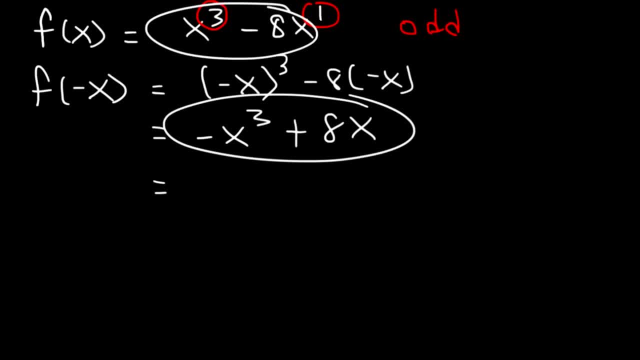 So now notice that all signs change. So to verify that it's odd, take out a negative 1.. If we factor out a negative 1, it's going to be positive x cubed. Negative 1 minus 8x. 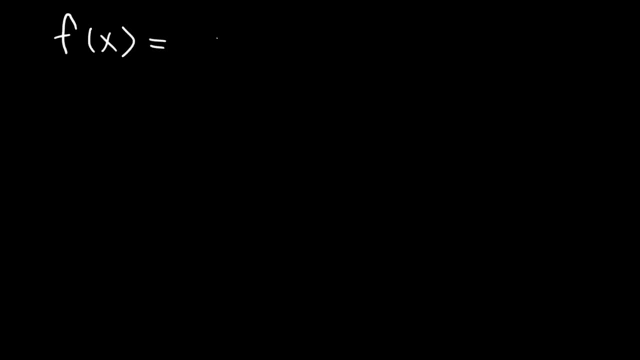 Now, what about this one? Let's say that f of x is equal to x squared plus 6.. Is it even or odd? Well, you know, x squared is an even component because it has an even exponent. What about 6?? Well, 6 is the same as 6x to the 0.. 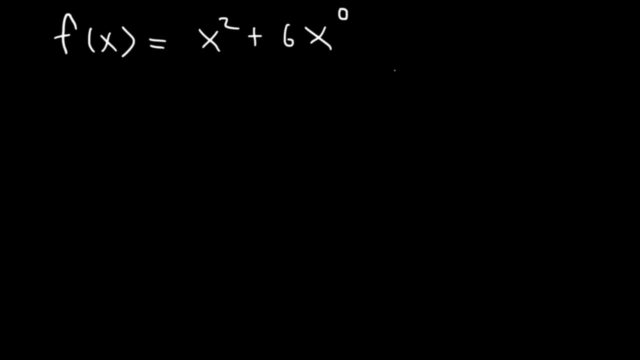 Anything raised to the 0, power is 1.. So x to the 0 is 1, which 6 times x to the 0 is 6 times 1 at 6.. And 0 is an even exponent, So the whole thing is going to be even. 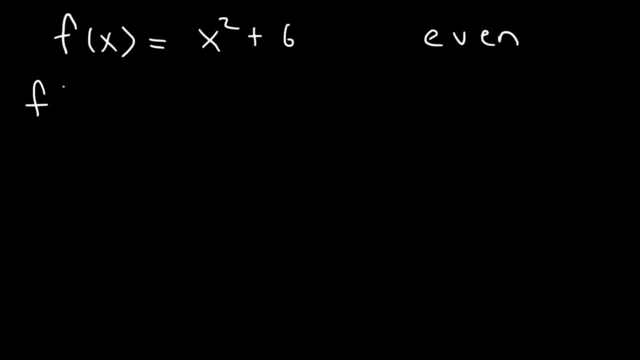 So let's go ahead and prove it Now. let's replace x with negative x, So this is going to be negative x squared plus 6.. Negative x times negative x is positive x squared, so we have x squared plus 6.. Notice that the function did not change. 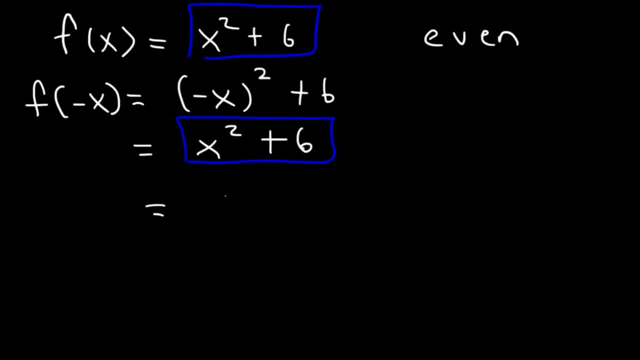 So on the right side we can replace x squared plus 6 with f of x. On the left side we still have f of negative x. So whenever f of negative x is equal to positive f of x, then it's an even function. 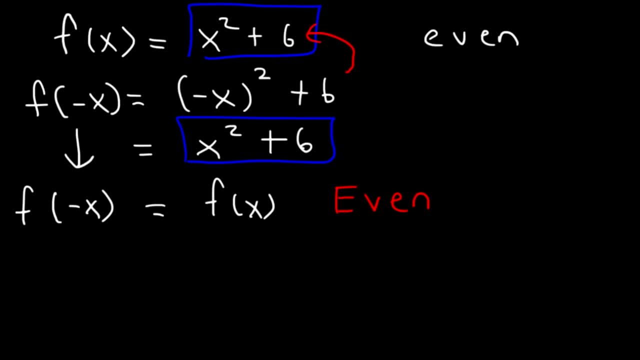 So if you see a number, it's even Think of that number as being multiplied times x to the 0.. And 0 is an even number, like 2, 4, 6.. What about x cubed minus 8x? 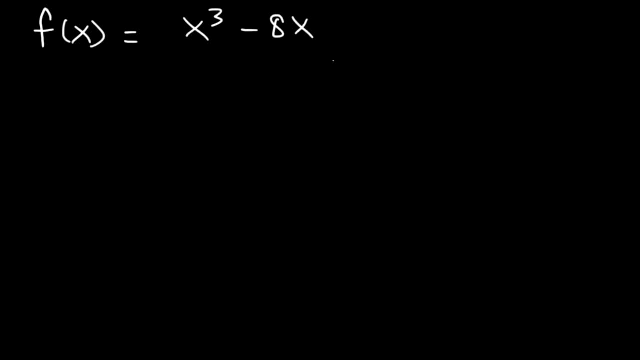 Is that even or is it odd? Well, whenever you see an x, it's basically x to the first power. Now, 1 is equal to x squared minus 8x. Now, 1 is equal to x squared minus 8x. 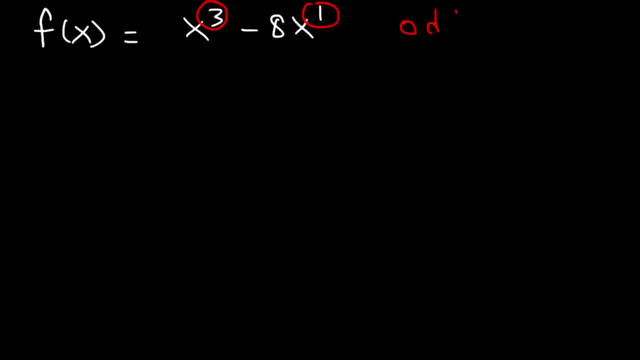 Now, 1 is equal to x squared minus 8x, And 3 are odd numbers, so therefore this is going to be an odd function. Now let's prove it. So let's find f of negative x. This is negative x to the third power. 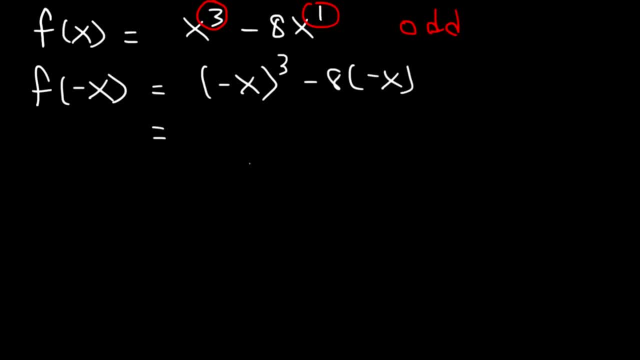 minus 8 times negative x Negative x to the third power is negative x cubed Negative 8 times negative. x is positive 8x. So now notice that all signs change. So to verify that it's odd, take out a negative 1.. 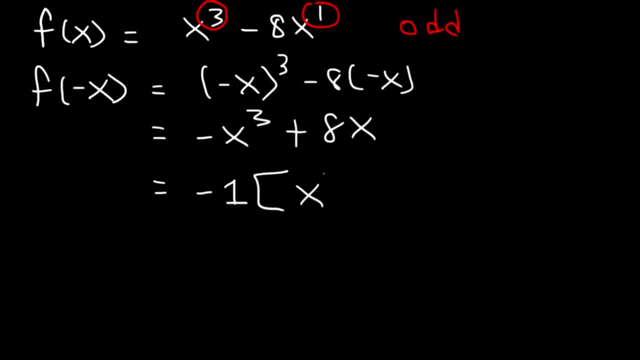 If we factor out a negative 1, it's going to be positive x cubed minus 8x And, as we can clearly see, x cubed minus 8x is basically the same as f of x. So therefore, f of negative x is equal to f of x. 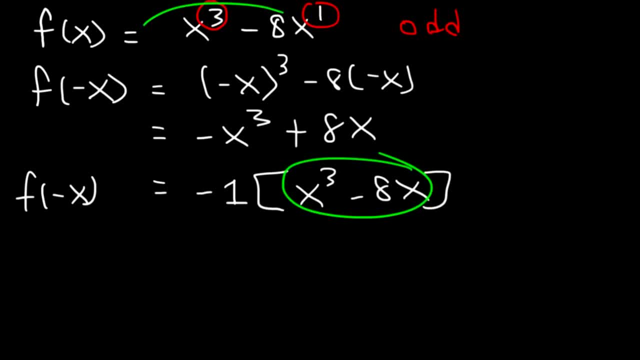 And, as we can clearly see, x cubed minus 8x is basically the same as f of x. So therefore, f of negative x is equal to f of x, which means that it's an odd function. Now, what about this example? 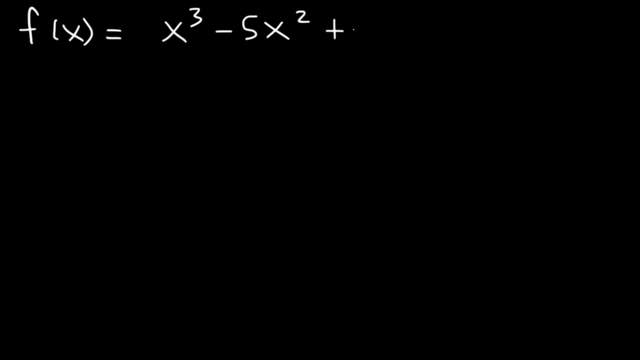 X to the third minus 5x squared plus 2.. Is it even or is it odd? It's even, It's odd. So notice that 3 is an odd exponent. 2 is an even exponent. Whenever you see even and odd exponents together, you know that it's going to be neither. 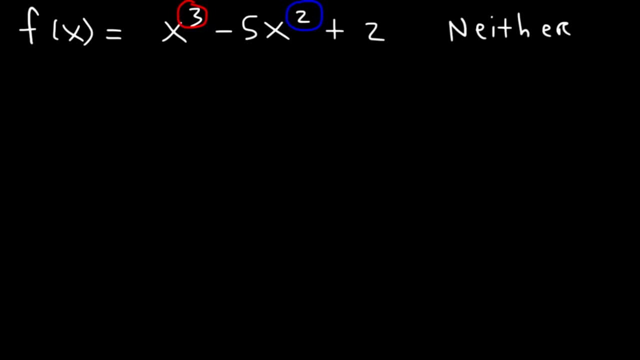 It's not even or odd. So that's how you can tell when it's neither, but let's prove it. So let's plug in negative x, Negative x to the third power minus 8 times negative x cubed is negative x cubed. 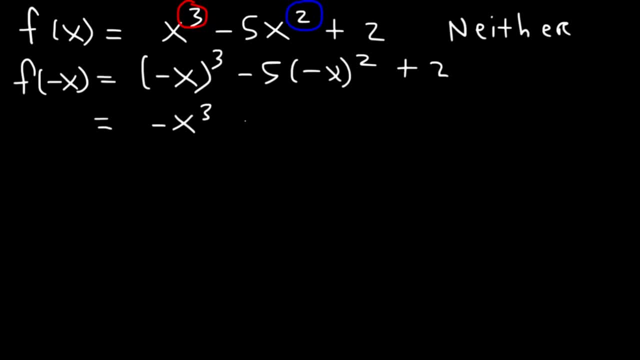 Negative x to the third power is negative x cubed And negative x to the second power is positive x squared. So this is what we have Now. let's check to see if it's an even function. If it's an even function right now, the original function should be the same as the new function. 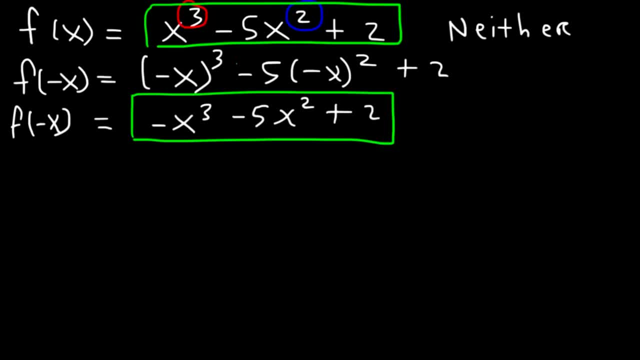 But notice that it's not the same. The sign for x cubed changed, But the sign for x squared No, And for 2, it did not change. So therefore it's not the same as the original function. So we can make the statement: f of negative x does not equal f of x. 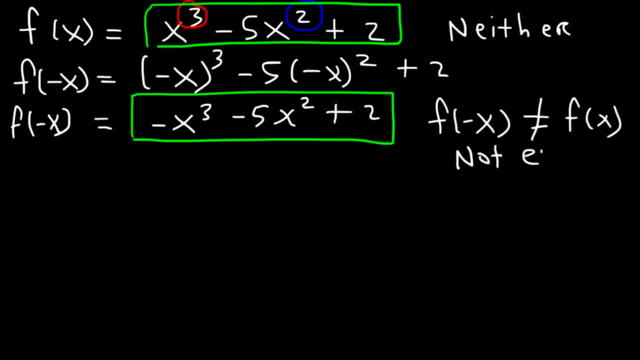 It's not even Now to check to see if it's an odd function. we need to take out or factor out a negative one. So all the signs will change. Negative: x cubed will become positive x cubed. Negative- 5x squared will become positive 5x squared. 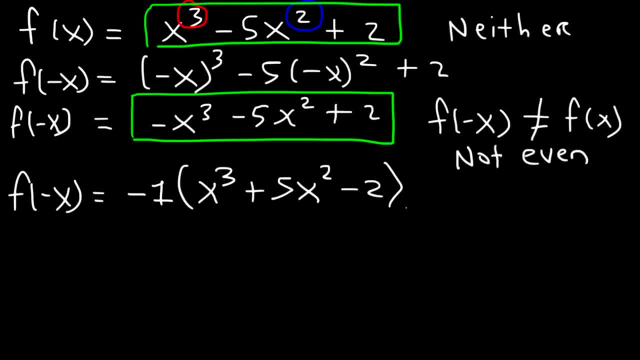 And 2 will become negative 2.. Now do we have the same function as the original function. Notice that these two are not the same. X cubed looks very similar. However, negative 5x squared is not the same as 5x squared. 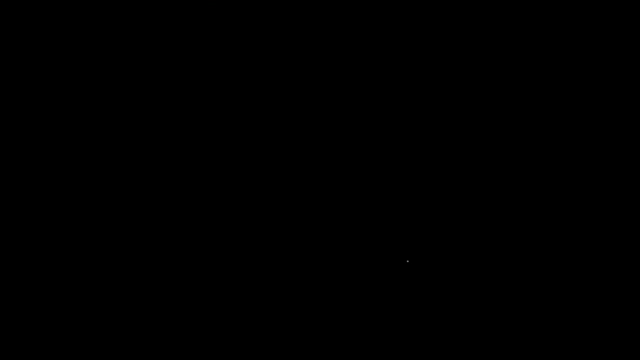 which means that it's an odd function. Now what about this example? x to the third, Minus 5x squared plus 2.. Is it even or is it odd? So notice that 3 is an odd exponent, 2 is an even exponent. 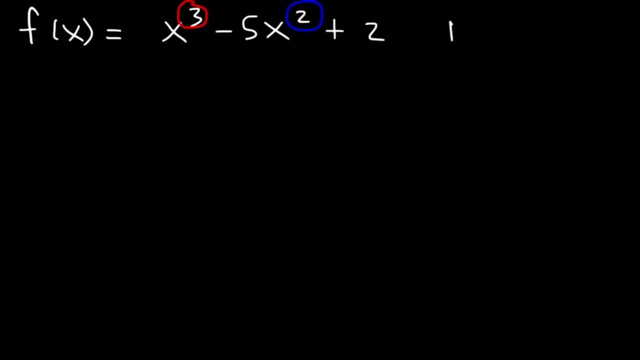 Whenever you see even and odd exponents together, you know that it's going to be neither. It's not even or odd. So that's how you can tell when it's neither. but let's prove it. So let's plug in negative x. 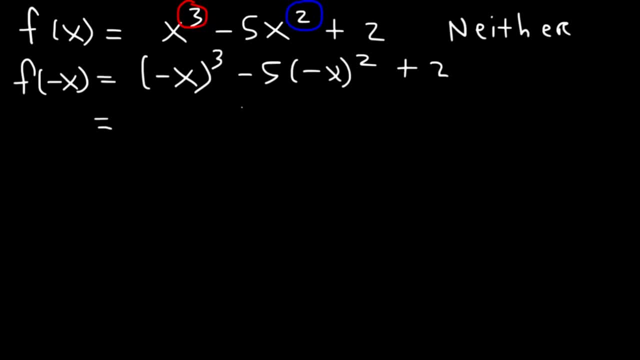 Negative x to the third power is negative x cubed And negative x to the second power is positive x squared. So this is what we have Now. let's check to see if it's an even function. If it's an even function. 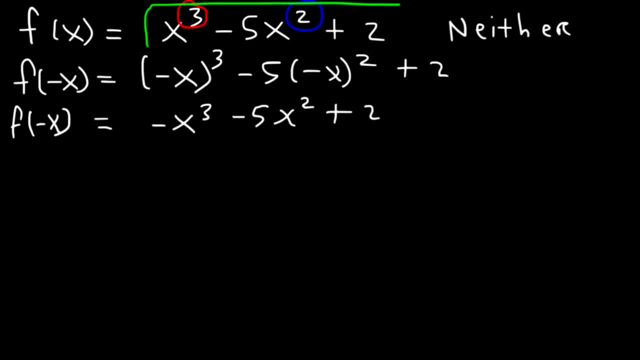 right now. the original function should be the same as the new function, But notice that it's not the same. The sign for x cubed changed, But the sign for x squared and for 2 did not change, So therefore it's not the same as the original function. 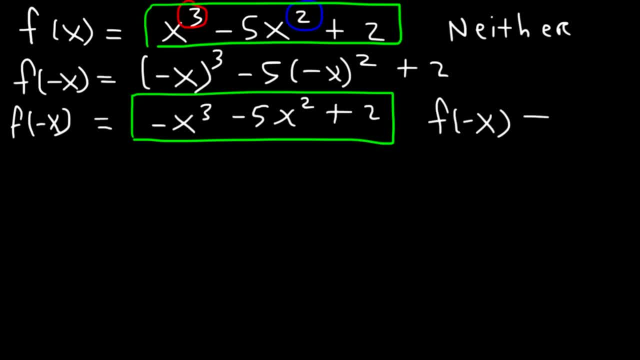 So we can make the statement: f of negative x does not equal f of x. It's not even Now to check to see if it's an odd function. we need to take out or factor out a negative 1.. So all this is an odd function. 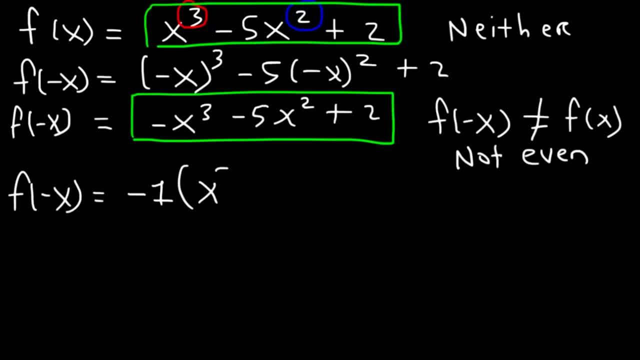 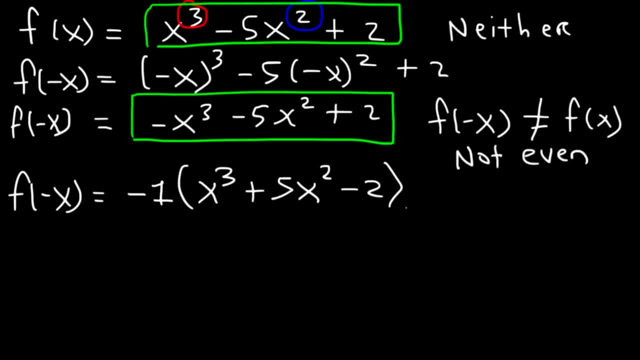 And 2 will become negative 2.. Now do we have the same function as the original function. Notice that these two are not the same. x cubed looks very similar. However, negative 5x squared is not the same as 5x squared. 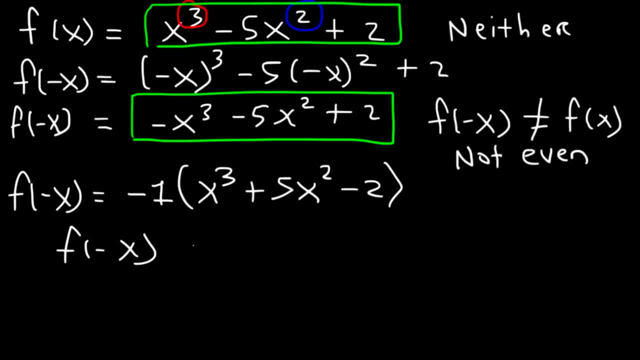 So therefore we can say that f of negative x is the same as 5x squared. Now the way it should beCoincidence is that an odd function does not equal negative f of x, but it becomes, even if it's not odd. 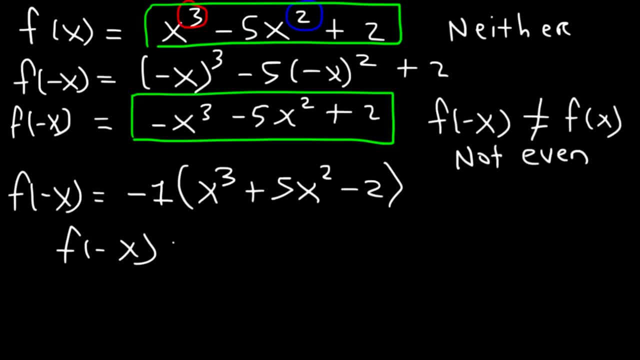 So therefore we can say that f of negative x does not equal negative x, Which means that it's not an odd function. So if it's not even and if it's not odd, then by default it has to be neither. So that's how you can prove if it's neither. 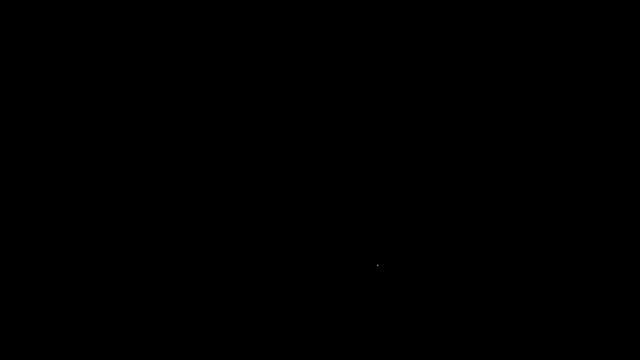 Now let's spend a few moments talking about graphs. An even function will be symmetric about the y-axis. An odd function is symmetric about the origin, And if it's not symmetric about the y-axis, then it's not even So. let's take a look at x squared. 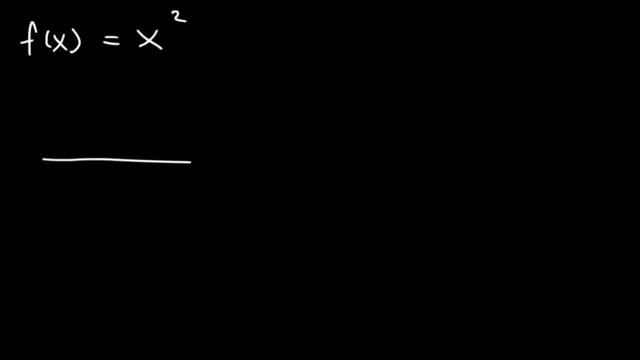 Because it has an even exponent. we know it's an even function. The graph of x squared looks like this: It's basically a u. Let's do that again. It's an upward u. Notice that there's symmetry about the y-axis. 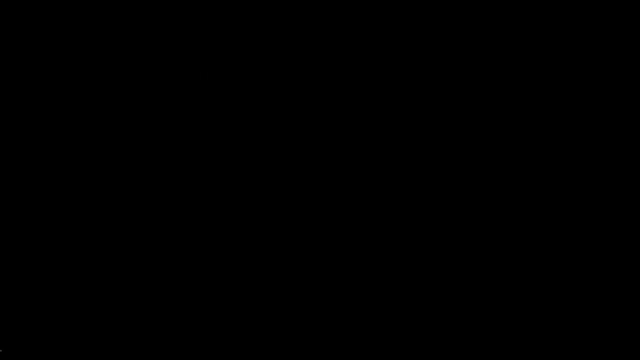 So that means that it's an even function. Now, if you have a constant, let's say like 3, that's an even function. f of x is the same as y. by the way, If you were to plot, y equals 3, it's going to be a horizontal line at 3.. 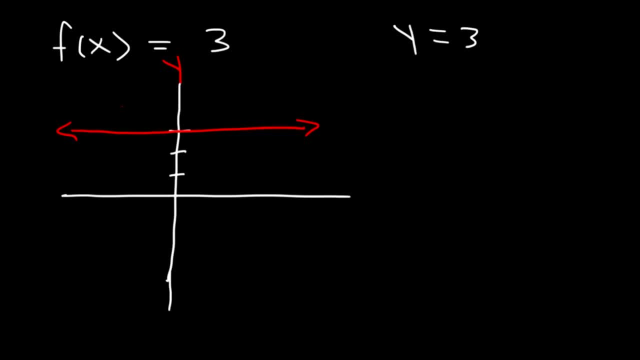 And notice that this line is symmetric about the y-axis: The left side looks exactly the same as the right side. So therefore, a constant, by definition, has even properties. Now let's take a look at x: squared, It's an even function. 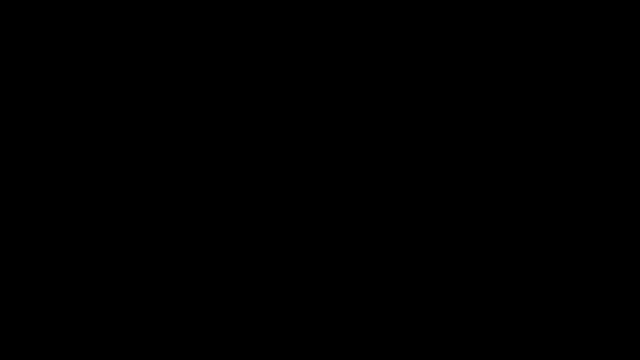 And notice that there's symmetry about the y-axis: The left side looks exactly the same as the right side. So therefore a constant by definition has even properties. Now what about the graph x cubed or y equals x cubed? 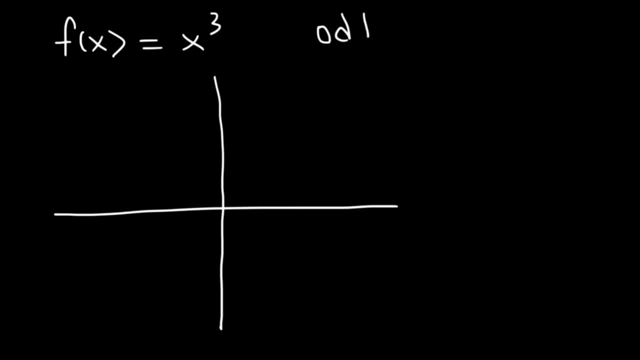 We know it's an odd function. This graph is an increase in function and it looks like this. As you can see, there's symmetry about the origin. This side in quadrant 1 looks exactly the same or it looks like a mirror image of the. 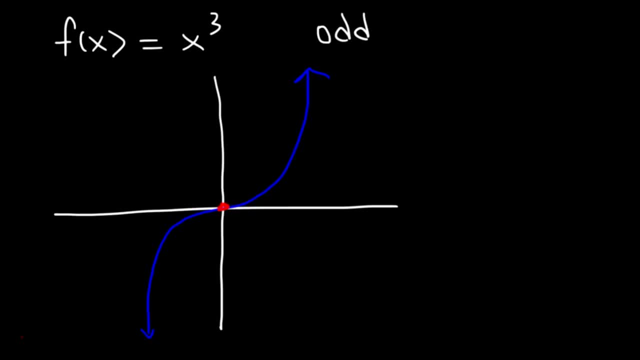 other side in quadrant 3.. So that's an example of an odd function. It's symmetric about the origin. And then there's the graph f of x equals x or y equals x to the first power. One is an odd number. 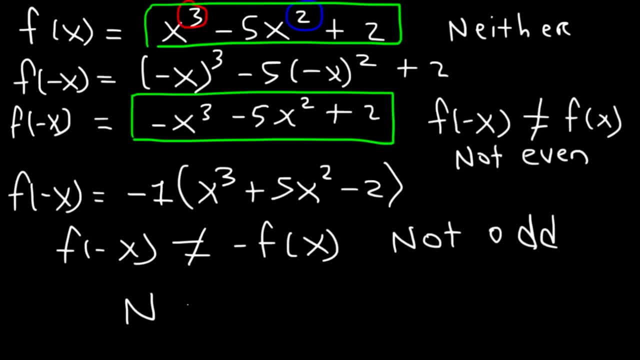 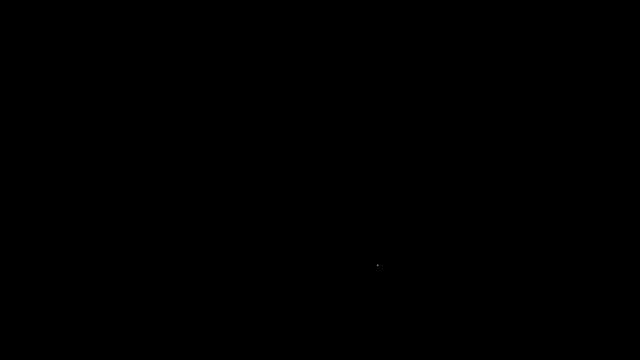 So if it's not even, and if it's not odd, then by def Sullivan, it has to be neither. So that's how you can prove If it's, and that An odd function is symmetric of the origin. An odd function is symmetric of 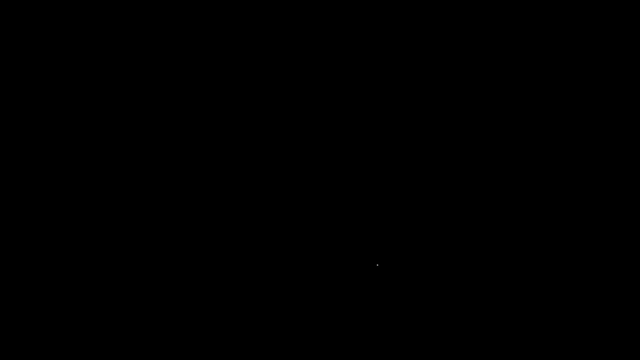 the source of our name. one. And if it's not symmetric about the origin or about the y-axis, then it's neither. So let's take a look at x squared, Because it has an even exponent. we know it's an even function. 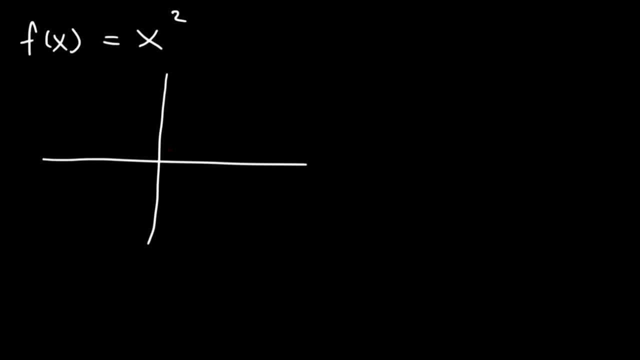 The graph of x squared looks like this: It's basically a u. Let's do that again. It's an upward u. Notice that there's symmetry about the y-axis, So that means that it's an even function. Now, if you have a constant, let's say like 3, that's an even function. 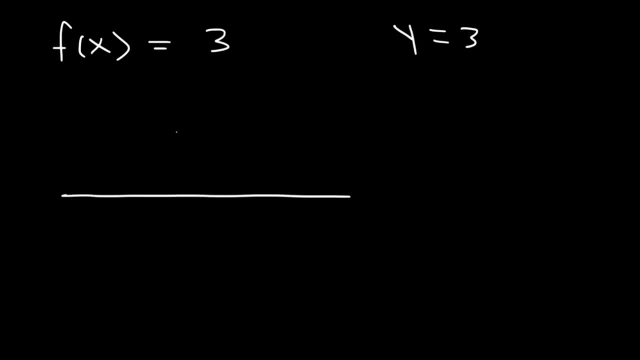 f of x is the same as y. by the way, If you were to plot, y equals 3, it's going to be a horizontal line at 3.. And notice that this line is symmetric about the y-axis. The left side looks exactly the same as the right side. 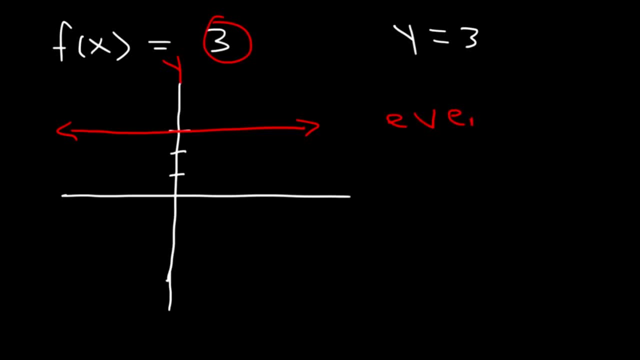 So therefore, a constant by definition has even properties. Now, what about the graph? x cubed or y equals x cubed? We know it's an odd function. This graph is an increase in function. It looks like this: 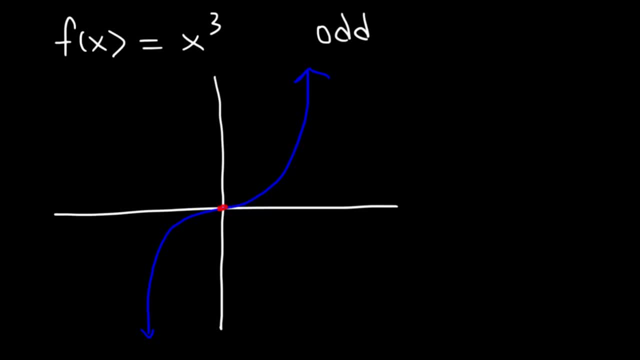 As you can see, there's symmetry about the origin. This side in quadrant 1 looks exactly the same, or it looks like a mirror image of the other side in quadrant 3.. So that's an example of an odd function. 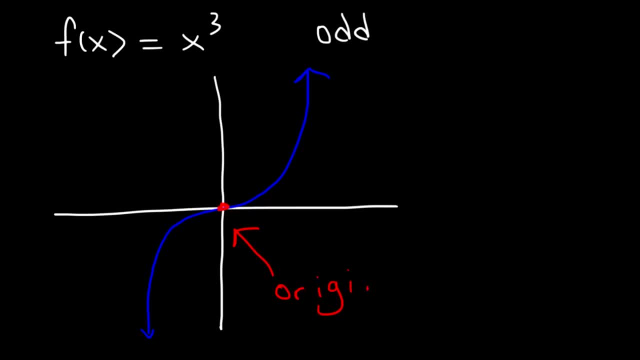 It's symmetric about the origin. And then there's the graph f of x equals x or y equals x. to the first power, 1 is an odd number. But let's see why this function is odd using a graph. So y equals x is basically a line that increases at a 45-degree angle. 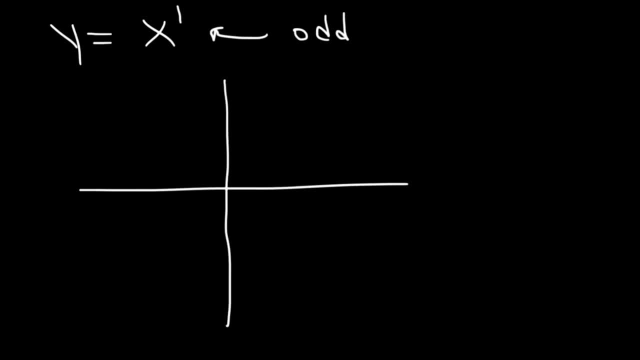 But let's see why this function is odd using a graph. So y equals x, is basically a line that increases at a 45 degree angle And, as you can see, it's symmetric about the origin. So that's an example of an odd function. 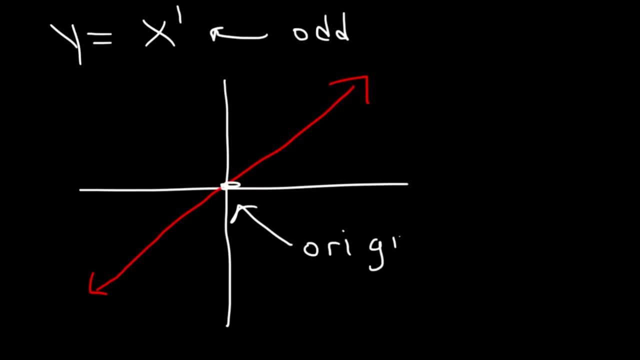 It's symmetric about the origin. The side in quadrant 1 looks like the same as the one in quadrant 3.. So there's symmetry about the origin, which is a property of an odd function. How would you describe a function that looks like this? 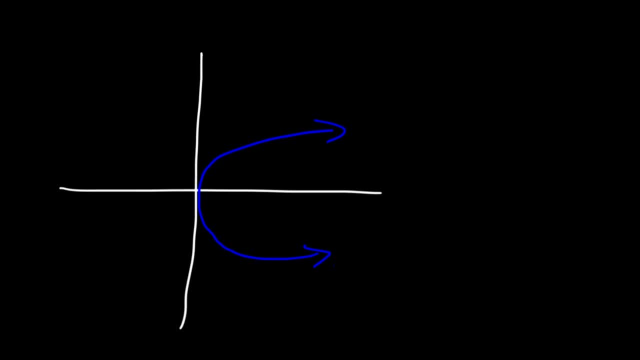 Is it even odd or neither? Now, here there's no symmetry about the y-axis or the origin, So this is neither. Now, what about this one? Is it even odd, or neither? Notice that the left side looks the same as the right side? 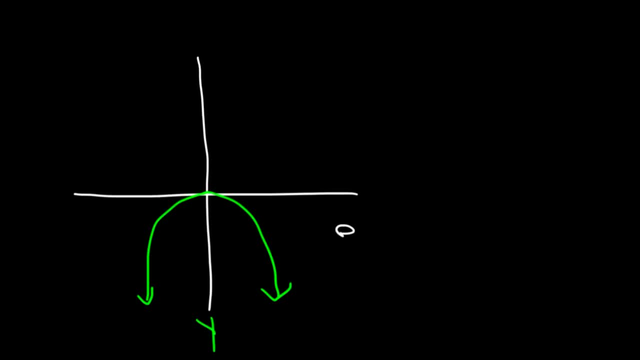 So therefore, it's symmetric about the y-axis, which means that it's an even function. Now, what about this one? Is it even, odd or neither? Here's another example for you. Determine if this one is even or if it's odd, or if it's neither. 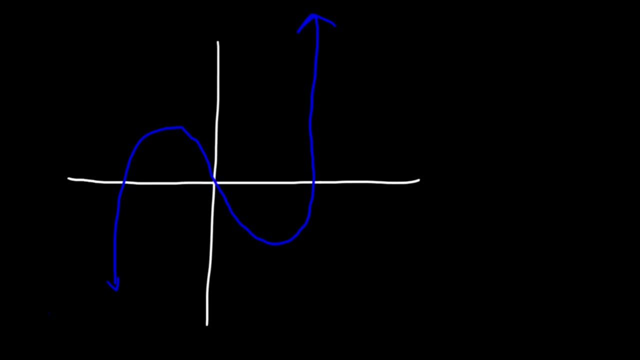 Now, it's not drawn perfectly to scale, so use your good judgment. So what would you say? Is it even odd, or neither Is it symmetrical about the y-axis- the origin, or neither It's not symmetric about the y-axis. 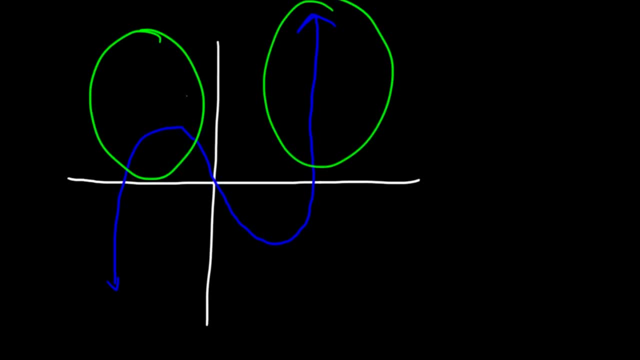 The right side does not look the same as the left side. However, there is symmetry about the origin. Notice that quadrant one looks similar to quadrant three. Now, this blue line could keep on going down, So, even though the height doesn't seem the same, it can keep going in that direction. 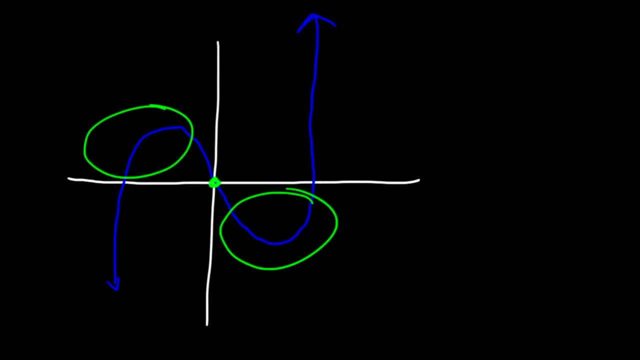 And notice that quadrant four looks like a reflection of quadrant two. As you can see, there's symmetry about the y-axis. So what would you say? Is it even odd, or neither? Here's another example. Note that quadrant two looks similar to quadrant three. 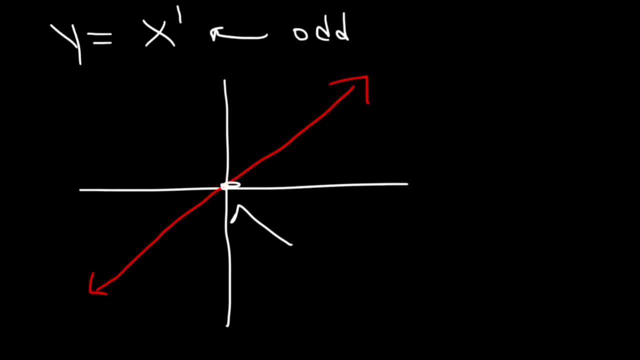 And, as you can see, it's symmetric about the origin. The side in quadrant 1 looks like the same as the one in quadrant 3.. So there's symmetry about the origin, which is a property of an odd function. How would you describe a function that looks like this? 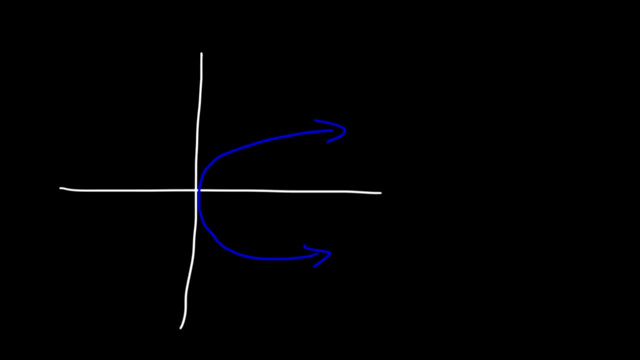 Is it even Odd Or neither? Now, here there's no symmetry about the y-axis or the origin, So this is neither. Now, what about this one? Is it even odd, or neither? Notice that the left side looks the same as the right side? 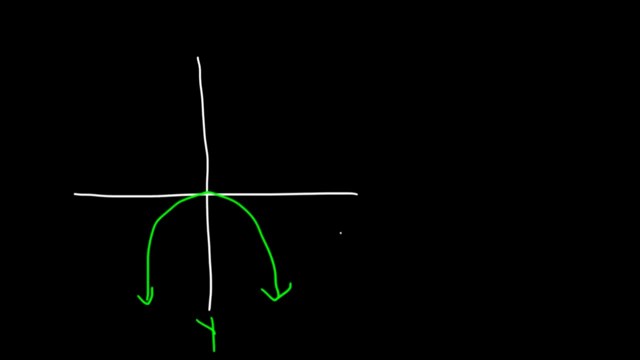 So therefore, it's symmetric about the y-axis, Which means that it's an even. Now what about the right side, Which means that it's an even function. Here's another example for you. Determine if this one is even or if it's odd. 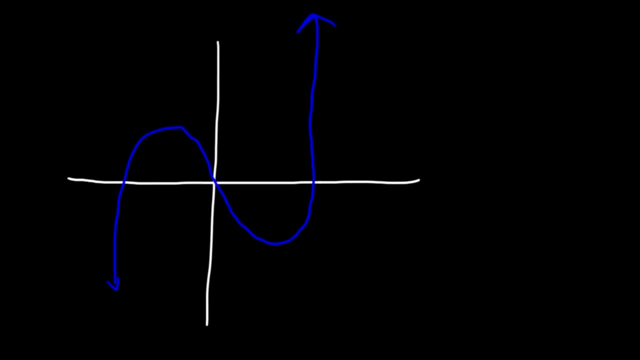 Or if it's neither. Now, it's not drawn perfectly to scale, so use your good judgment. So what would you say? Is it even odd or neither? Is it symmetrical about the y-axis, the origin, or neither? 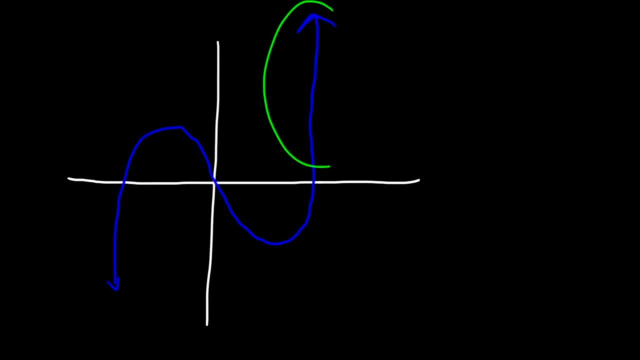 It's not symmetric about the y-axis: The right side does not look the same as the left side. However, there is symmetry about the origin. Notice that quadrant 1 looks similar to quadrant 3.. Now this blue line could keep on going down. 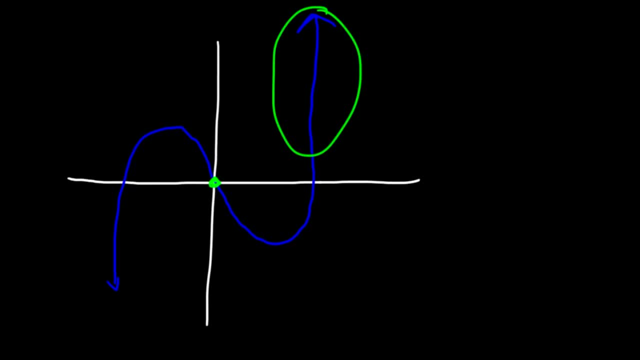 So, even though the height doesn't seem the same, it can keep going in that direction. Notice that quadrant 4 looks like a reflection of quadrant 2.. As you can see, there's symmetry about the origin, which makes this function an odd function. 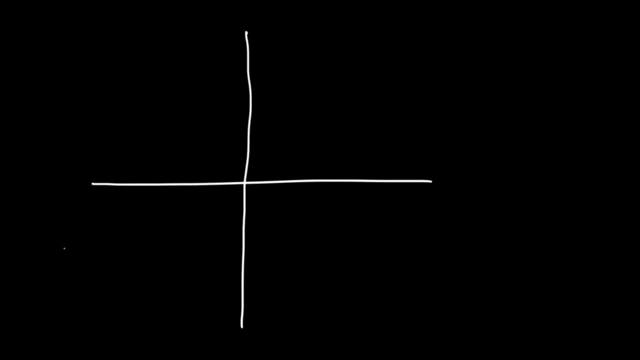 Here's another one for you. Is it symmetric? Is this an even or is it an odd function? So notice that the right side looks the same as the left side. Therefore, it's an even function. It's symmetric. about the y-axis: 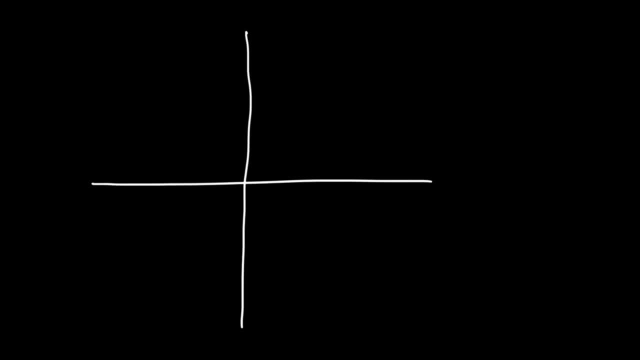 Note that the right side is like a circle and the left side is a vertical rectangle. So even though the height doesn't seem the same, it's symmetrical about the y-axis. Notice that quadrant two looks like a vertical rectangle. So even though the height doesn't seem the same, it's symmetrical about the y-axis. 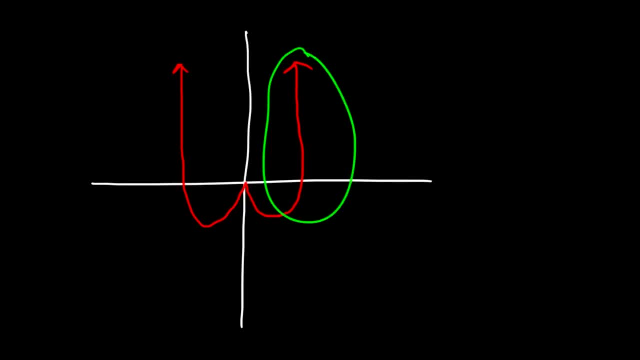 Note that quadrant three looks like a rectangle. It looks the same as the left side. Therefore it's an even function. It's symmetric about the y-axis. And what about this example? Is it even odd or is it neither? 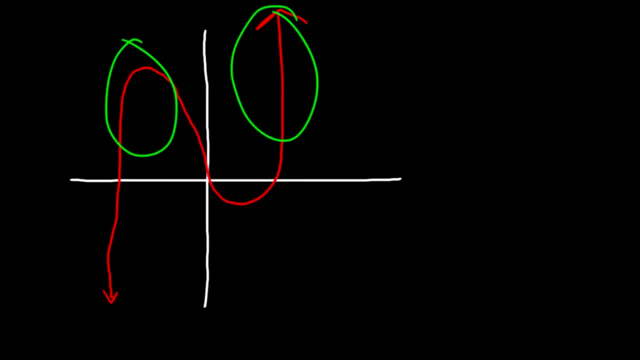 Well, we know it's not. even The right side does not look the same as the left side, And it's not odd. Now you can clearly see a difference between this section and this section. It's not symmetric about the origin. 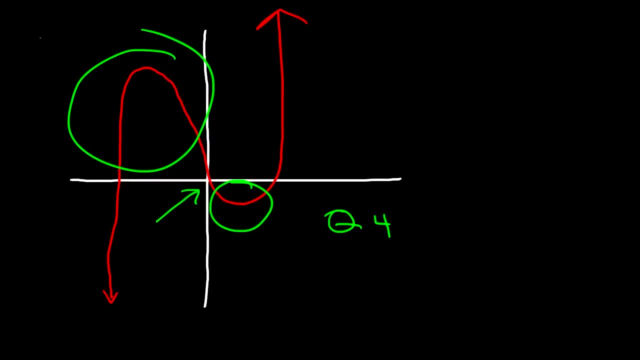 Because quadrants 4 and quadrant 2 doesn't have the symmetry about the origin. They don't look the same. So in this case this function will be neither. It's neither even, nor is it odd. Let's try one more example. 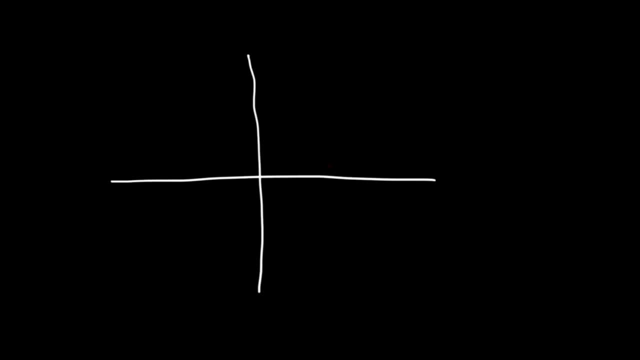 Now what if we have, let's say, a circle? Let me draw a better circle. It's not perfect, but let's say it's a well-rounded circle. Is it even odd, or neither? Well, the circle does have even properties. 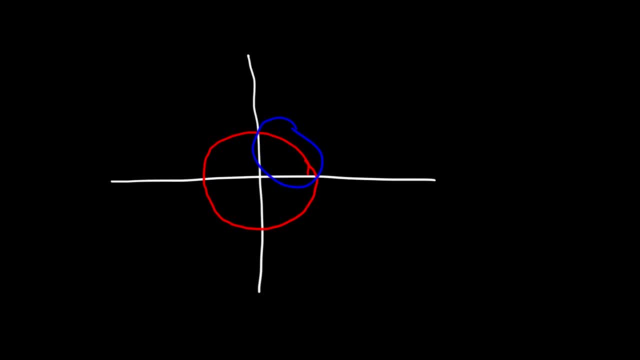 As you can see, the right side looks the same as the left side. This whole side looks the same as the left side. This whole side looks the same as the left side. They're the same. So there is symmetry about the y-axis. 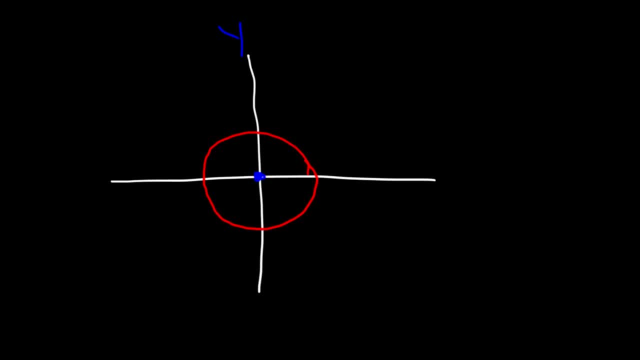 Now, what about the origin? Is it symmetric about the origin? What would you say? Notice that the side in quadrant 1 looks like a reflection as the one in quadrant 3.. So there's some symmetry about the origin, And quadrant 2 and 4 are symmetrical about the origin. 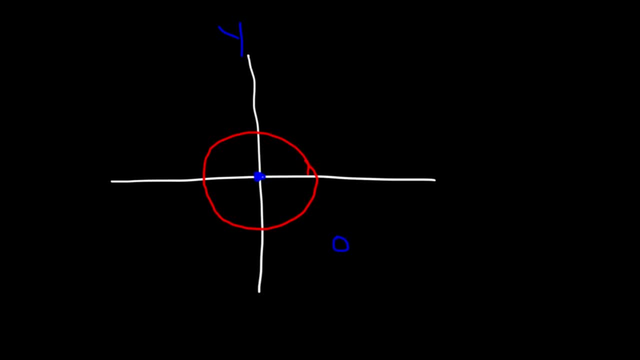 So this graph is symmetric about the y-axis And About the origin as well. So does that make it even or odd? Now, technically speaking, we can't really say it's even or odd because it's not a function. This function doesn't pass the vertical line test. 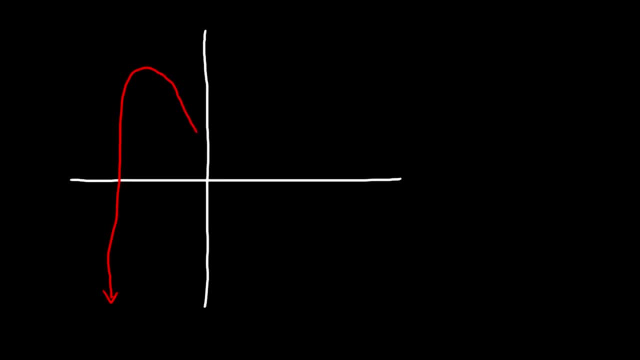 What about this example? Is it even, Is it odd, Or is it neither? Well, we know it's not even. The right side does not look the same as the left side And it's not odd. You can clearly see a difference between this section and this section. 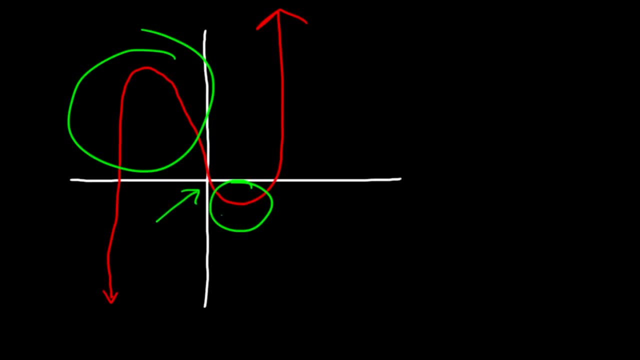 It's not symmetric about the origin, because quadrants 4 and quadrant 2 doesn't have the symmetry about the origin. They don't look the same, So in this case this function will be neither. It's neither even, nor is it odd. 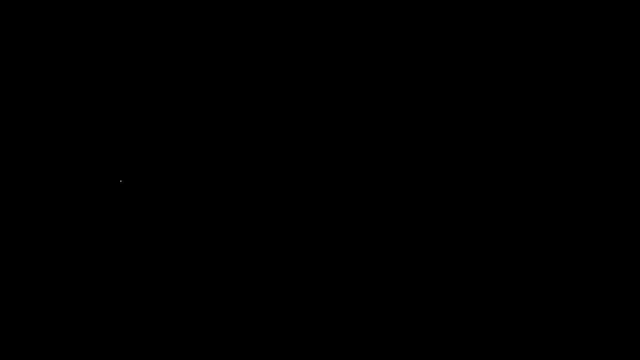 Let's try one more example. Now, what if we have, let's say, a circle? Let me draw a better circle. It's not perfect, but let's say it's a well-rounded circle. Is it even odd, or neither. 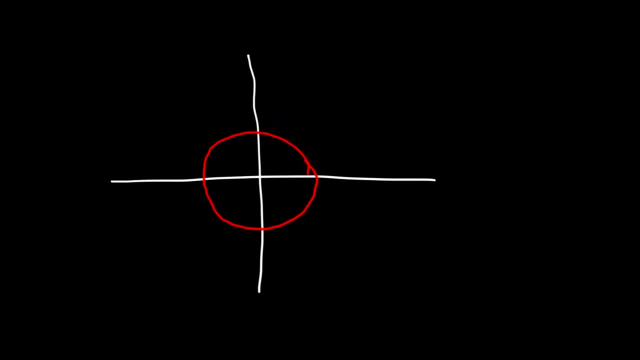 Well, the circle does have even properties, As you can see. the right side looks the same. It's symmetric. It doesn't look the same as the left side. This whole side did the same, So there is symmetry about the y-axis. 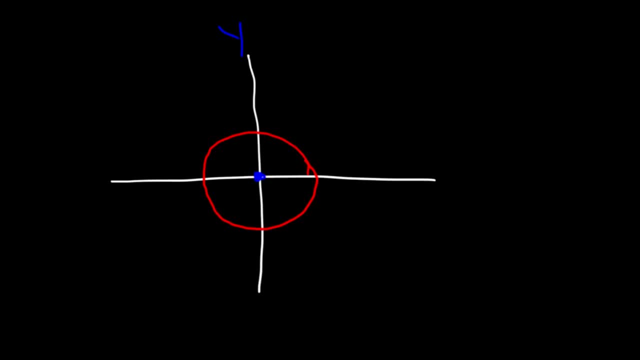 Now, what about the origin? Is it symmetric about the origin? What would you say? Notice that the side in quadrant 1 looks like a reflection as the one in quadrant 3.. So there's some symmetry about the origin, And quadrant 2 and 4 are symmetrical about the origin. 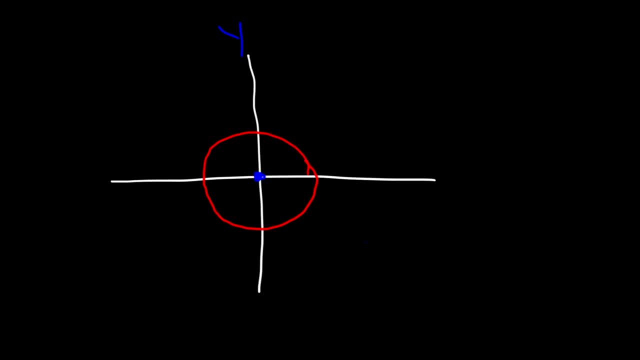 So this graph is symmetrical about the y-axis and about the origin as well. So does that make it even or odd? Now, technically speaking, we can't really say it's even or odd because it's not a function. This function doesn't pass the vertical line test. 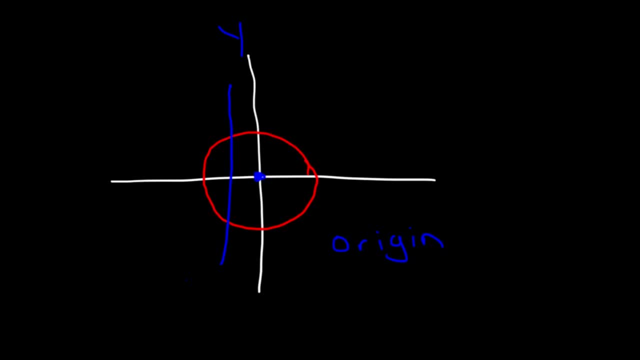 So we can't say it's an odd function, it's not an even function, Maybe it's neither, because it's not a function. So think about that one.